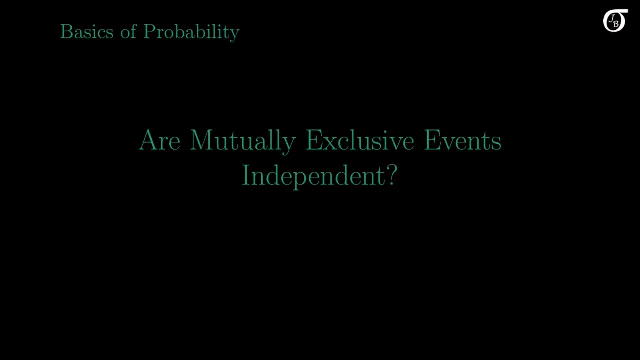 but I will do a very brief review of those concepts. Here's our formal definition of independence. Events A and B are independent if, and only if, the probability of the intersection is equal to the product of the individual probabilities. You might have seen independence defined in terms of conditional probabilities. 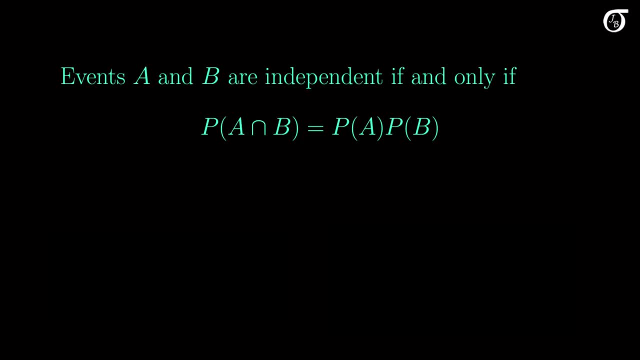 which leads to a more intuitive explanation and is a reasonable approach, but mathematically we run into a bit of a snag. Here's the conditional probability formula for event A given event B, but this is not defined if the probability of B is 0. 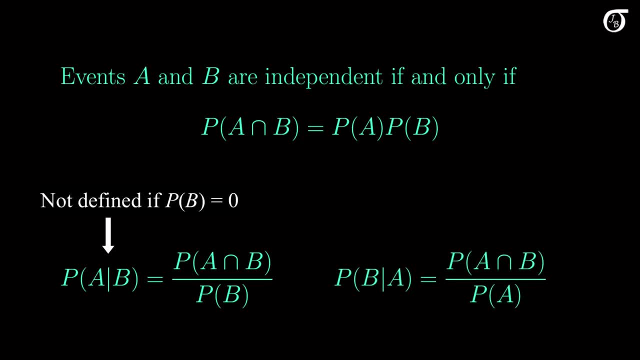 Similarly, here's the conditional probability formula for event B, given event A has occurred. but this is not defined if the probability of A is 0. So we run into snags in the zero probability case, and that zero probability case is meaningful for the problem we're looking at in this video. 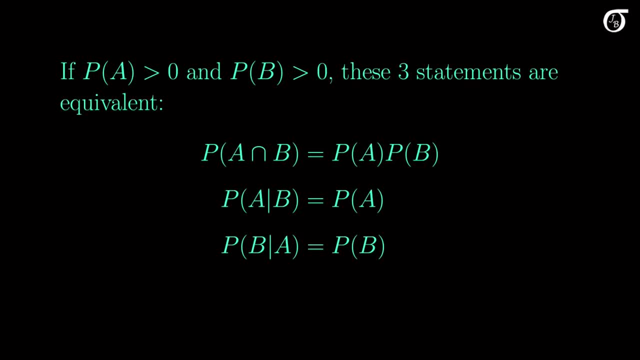 For the case where both probabilities are non-zero, these three statements are equivalent and they all mean that A and B are independent events. Each of these three statements implies the others. If one of these statements is true, then they are all true and A and B are independent. 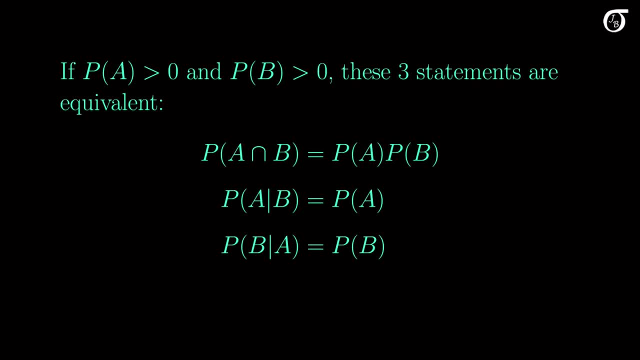 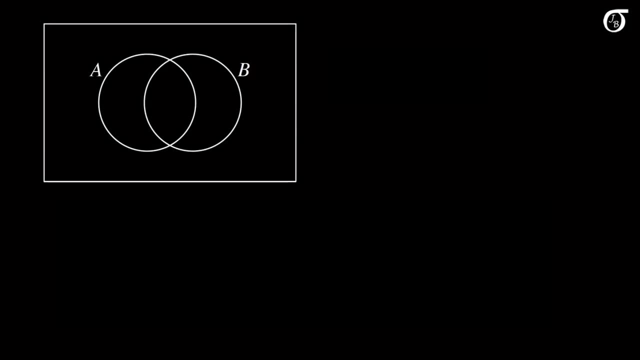 If one is false, they are all false, and A and B are not independent. Now to the problem. Here is a visual representation of events A and B. Here, visually at least, A and B share part of the sample space. And here is a visual representation of mutually exclusive events. 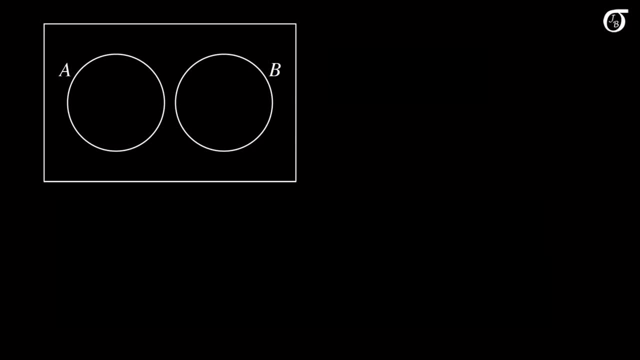 Here A and B share no common ground in the sample space. They share no sample points and they cannot occur together. Some students look at this and think that A and B are separate, that they're doing their own thing and so they're independent. 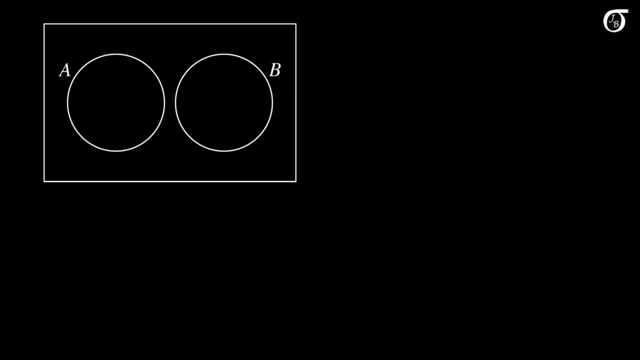 But that's not what independence means in a probability sense. Let's look at what this situation does tell us. Here the events are mutually exclusive, so the probability of their intersection is zero. But if the probability of the intersection is zero, that can only equal the product of the individual probabilities. 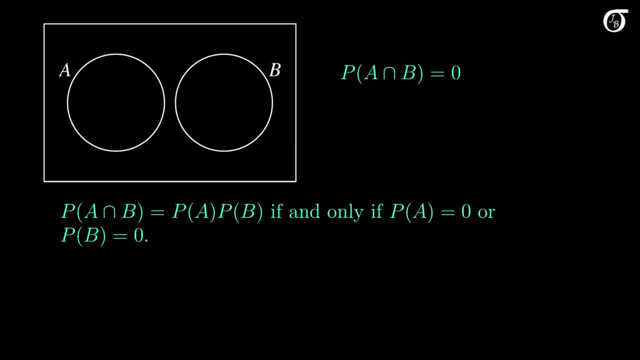 if the probability of A is zero or the probability of B is zero, or both are zero. So if A and B are mutually exclusive events, they are independent if, and only if, the probability of A is zero or the probability of B is zero. 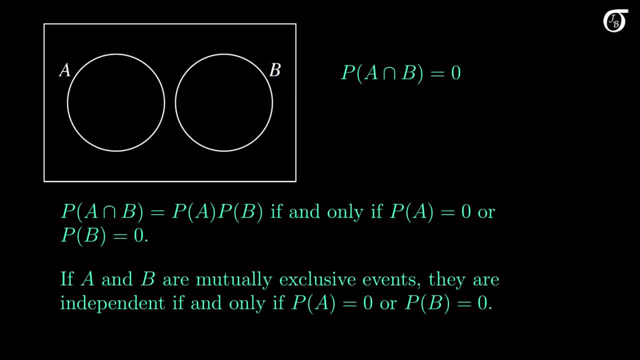 But I'm not particularly interested in this special case of zero probabilities in this situation, and I think that the case where A and B both have positive probabilities of occurring is a little more meaningful. So, at the risk of being a little redundant, I'm going to take a closer look at that scenario. 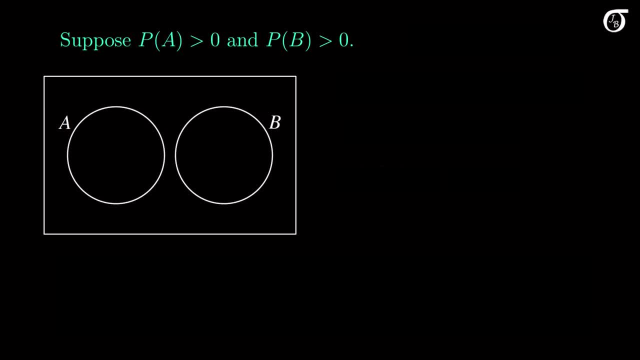 Suppose that A and B are mutually exclusive events, where the probability of A is greater than zero, as is the probability of B. This of course implies that the product of their probabilities is greater than zero. They are assumed to be mutually exclusive here, so the probability of their intersection is zero. 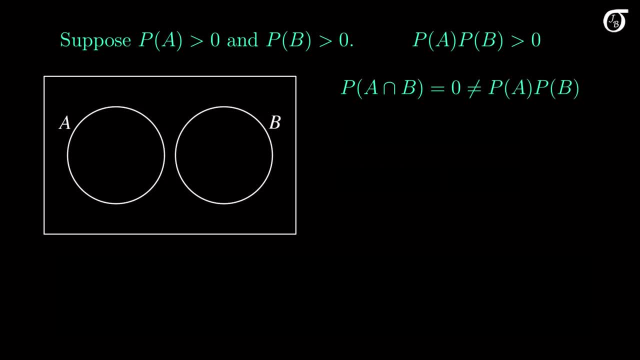 and thus the probability of their intersection is not equal to the product of their individual probabilities. This means that if A and B are mutually exclusive events with positive probabilities of occurring, then A and B are not independent. We could also phrase this in terms of conditional probability. 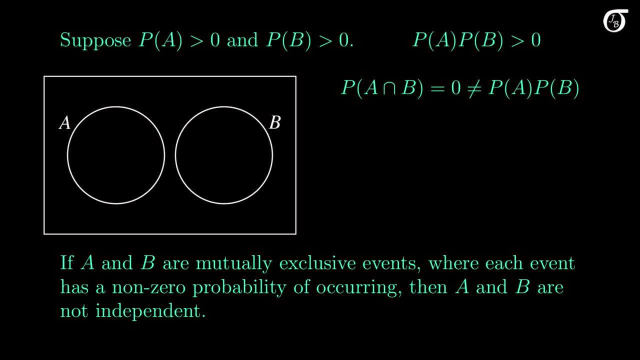 which might make a little more intuitive sense for some Here. if A happens, what is the probability of A? Well, if we're in circle B, we cannot be in circle A, so the probability of A given B is zero. You can verify that with the conditional probability formula if you wish. 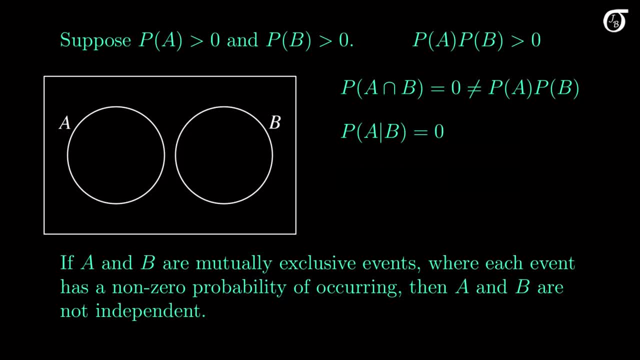 The original probability of A is greater than zero here. so the conditional probability of A given B is not equal to the probability of A, and thus A and B are not independent. The knowledge that B has occurred has changed the probability of A from a, whatever it was originally, to zero. 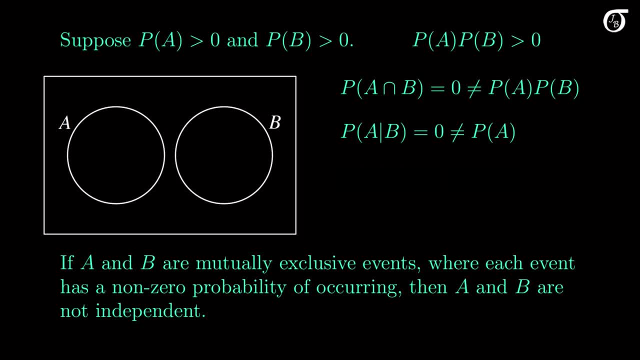 A and B are very much dependent And of course we could easily switch B and A around and make the same argument with the conditional probability of B given A. If we are in circle A, then we cannot be in circle B, and thus the probability of B given A is zero. 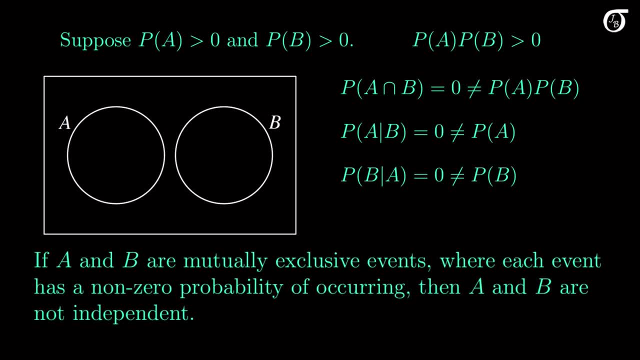 And we could have used any one of these three statements to draw this conclusion. Thank you for watching.